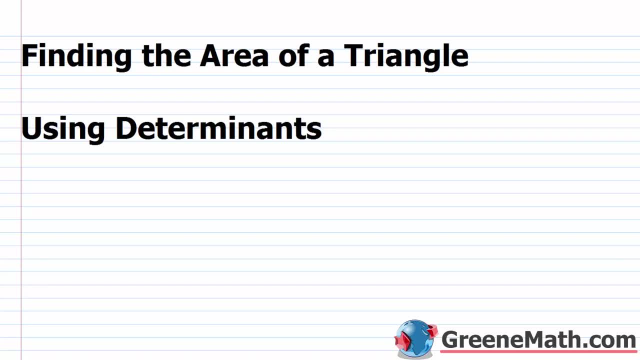 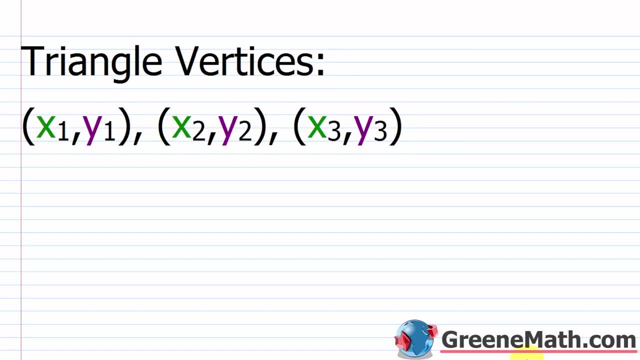 In this lesson we want to talk about finding the area of a triangle using determinants. All right, so an application of kind of matrices and determinants is being able to find the area of a triangle whose vertices are given as points in our coordinate plane. So you have these three. 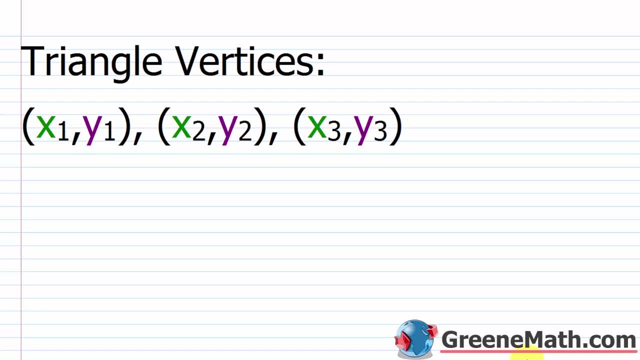 vertices that you're going to be given, and the first thing you want to do is you want to label: 1 is x sub 1, y sub 1,, 1 is x sub 2, y sub 2, and then, kind of, the last one is x sub 3, y sub 3.. 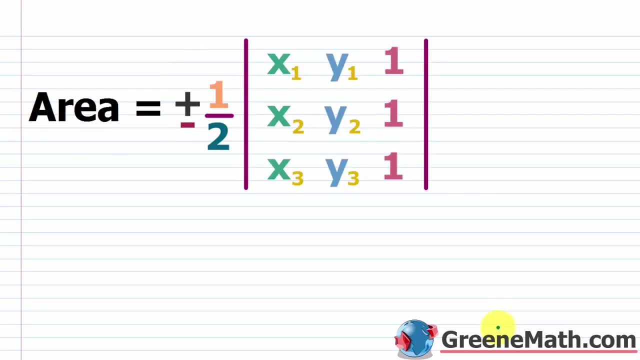 And the first thing you're going to ask me is: does it matter which point gets labeled as which? and it doesn't? Okay, and I'll explain why in a moment. So then you're going to plug into this kind of formula here for the area of a triangle. So you see, it's equal to you have plus or minus. 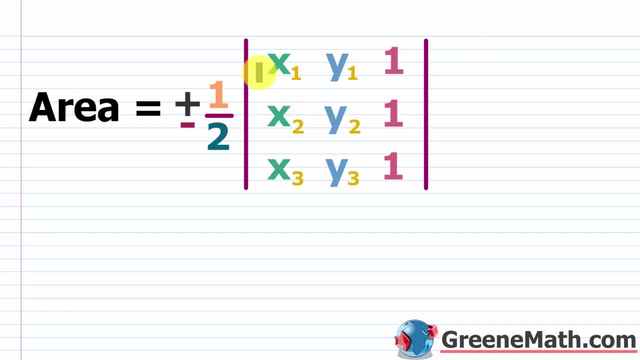 this one half times the determinant of this guy. Remember, if you see these vertical bars, it means to take the determinant. Okay, so, first and foremost, before I explain anything, just notice where you're plugging things in at. You've labeled stuff as x sub 1, y sub 1 through, x sub 3, y sub 3.. 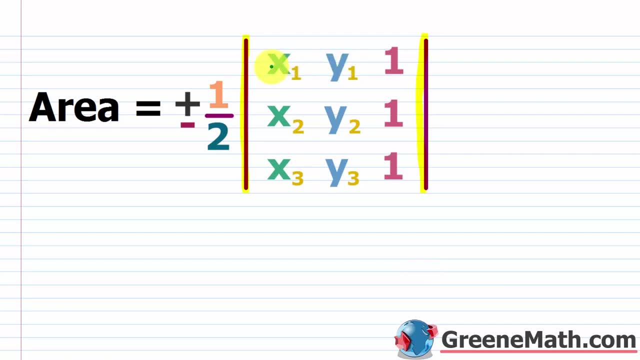 You're plugging in the area of a triangle and you're going to plug in the area of a triangle. So you're plugging in x sub 1, y sub 1 in this first row. So you have that there and there, okay, and then you always have a 1 in the third column. Then you're going to plug in x sub 2, y sub 2 always. 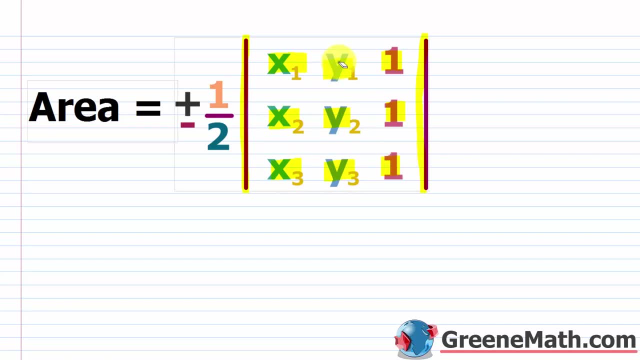 have a 1.. x sub 3, y sub 3- always have a 1.. Okay, so that takes care of that, and then you're going to take the determinant. Now this is where I need to start explaining things. So you have that plus, or? 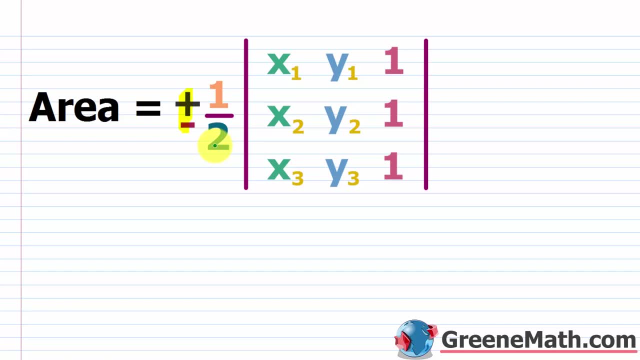 minus there. that might be super confusing for you and basically what this is telling us is that we want to make sure that we get a positive area. Okay, so if the determinant evaluates to be negative, you multiply by negative one half to get a positive area. If the determinant evaluates: 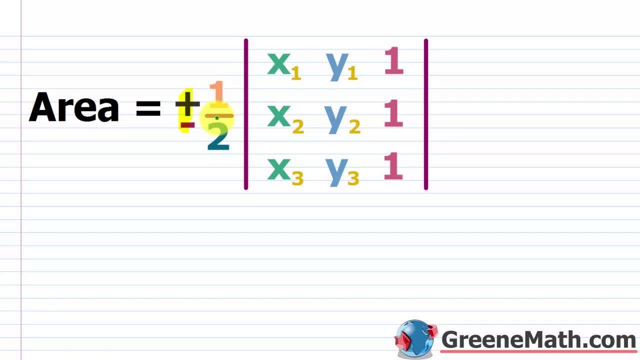 to be positive. well then I can just multiply by positive one half and again I get a positive area. Now the other scenario is you end up with an area that's zero, and we're going to talk about this specifically in the next lesson. If your area evaluates to zero the three points that you had, 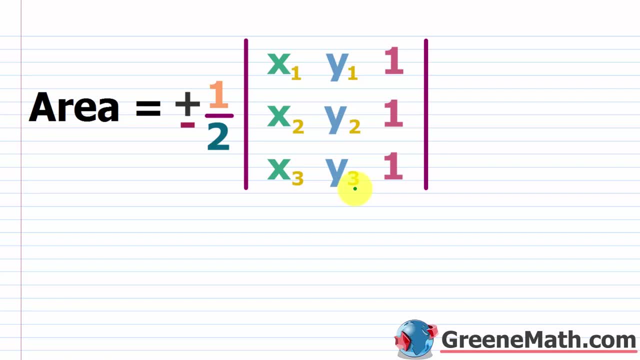 are actually on the same line. Okay, so that's going to be our test for collinearity, and we're going to talk about that specifically in the next lesson. For today we're just going to look at two problems, and neither is going to have an area of zero. So let's talk about the final question and 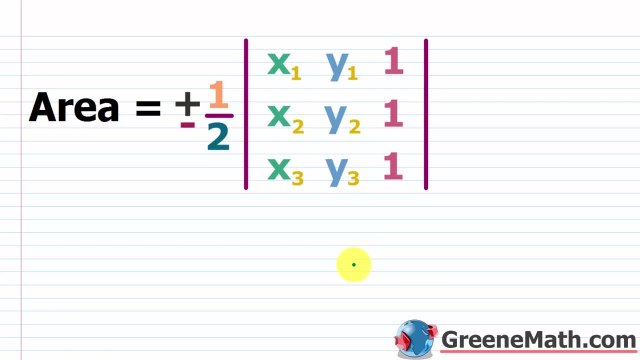 that's why am I able to label, you know, any of these as x sub 1, y sub 1, or x sub 2, y sub 2 or x sub 3, y sub 3.. Well, I don't have to go in a certain order. Well, it deals with the properties of. 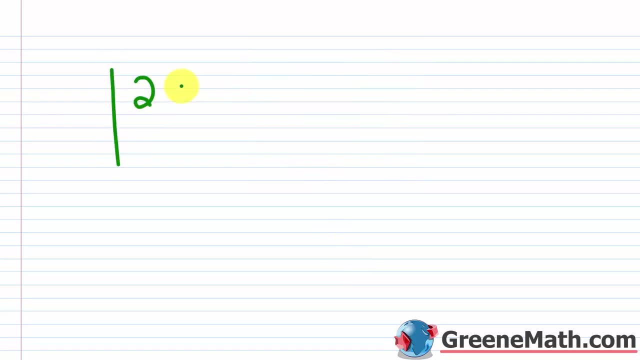 determinants that we've already talked about. If I had something like 2, 3, 4, 5, like this: the determinant is what 2 times 5 is 10 minus 3 times 4 is 12.. This is negative 2.. Okay, what happens if we swap rows? 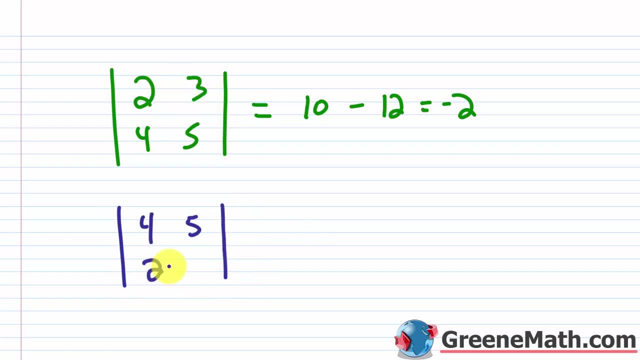 So let's say, I put the 4 and the 5 into row 1 and the 2 and the 3 in row 2.. Well, what happens is the sign of the determinant changes. right, The absolute value is the same. The absolute value will be 2 in. 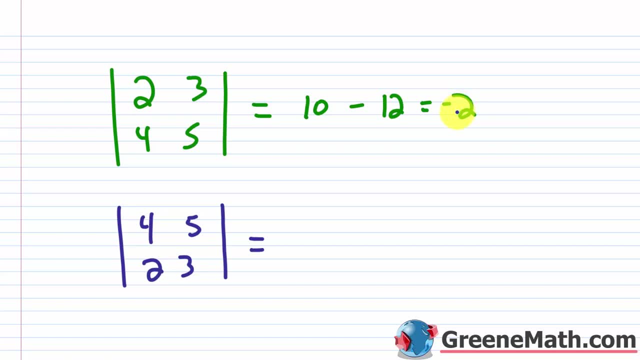 each case. but now, instead of getting a negative 2, I'm going to have a positive 2.. So 4 times 3 is 12, and then minus 5 times 2 is 10.. So this is going to be positive 2 versus the negative 2 there. 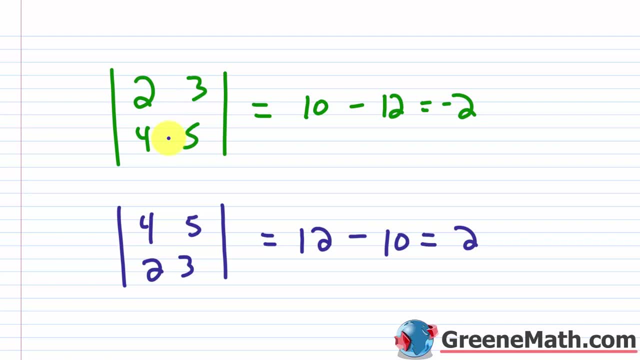 Okay, so when we swap rows, okay, we just change the sign. Now think about this here: If I had a certain configuration here, I've kind of labeled everything If one yields a positive, and then I switch what got labeled as kind of x sub 1, y sub 1 with what got labeled as x sub 2, y sub 2.. I'm 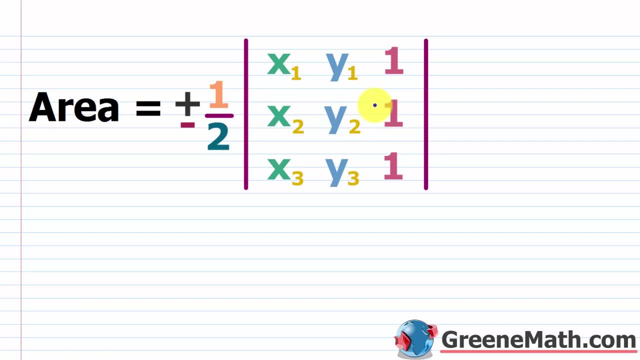 basically just swapping rows, So it's just going to change the sign of the determinant. The absolute value will still be the same and I have this plus or minus here to take care of any situation where I get a negative. So I'm good to go All right. so, with that being said, 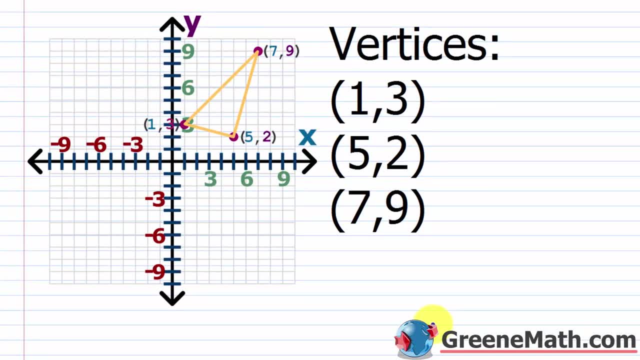 let's jump into the first example. And so we have this triangle with the following vertices. We have this: 1, 3, which is going to be this guy right here. okay, 1 units to the right, 3 units up. 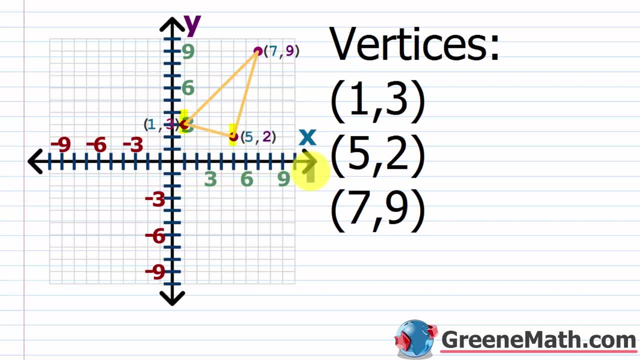 5, 2,- that's this guy right here- 5 units to the right, 2 units up. And then 7, 9,. so 7 units to the right, 9 units up. So right there. So those are our three vertices. 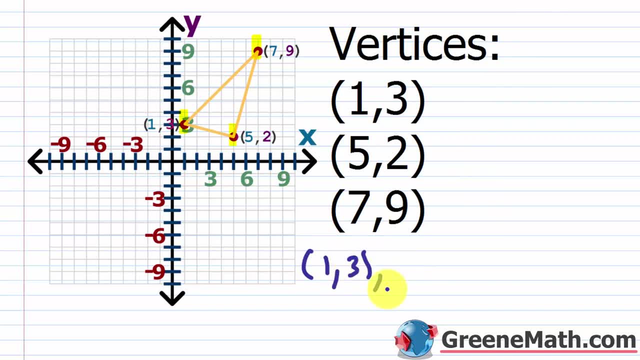 Let's just copy them real quick. So 1, 3, and then we have 5, 2, and then we have 7, 9.. Okay, so let's copy this and let's go back up And I'm just going to paste this in here real quick. 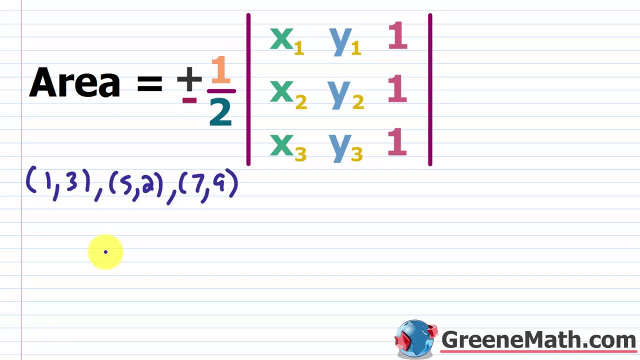 And we'll just kind of fill this out. We'll go to a fresh sheet because I don't think I can fit everything. So the area is equal to plus or minus 1 half times the determinant of this guy. So I'm just going to label these in order. 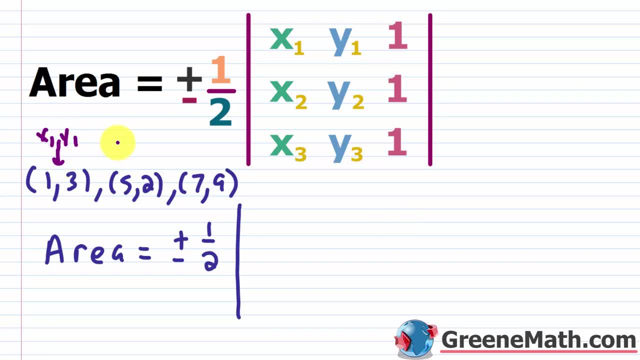 I'll just say this is x sub 1, y sub 1.. I'll say this is x sub 2, y sub 2.. And I'll say this is x sub 3, y sub 3.. And again, it does not matter what gets labeled as which. 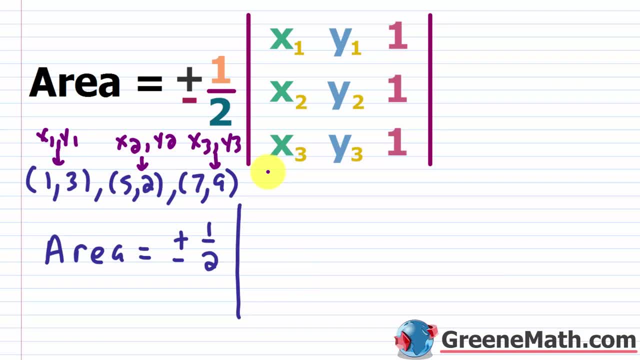 And just to prove that to you, I'll swap it after I do this. Okay, so I'm going to plug in a 1, a 3, and then I'll always have a 1.. Then I'm going to plug in a 5, a 2, and again I'll always have a 1.. 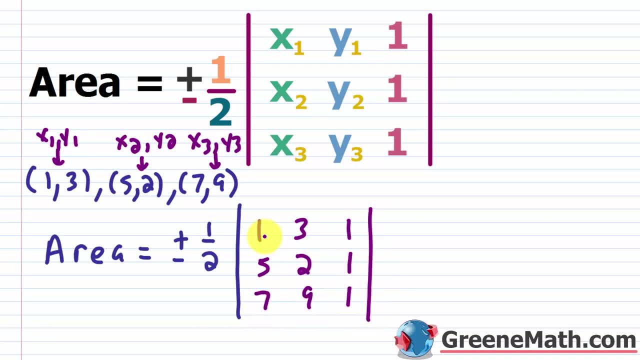 And then a 7,, a 9,, and I'll always have a 1.. Okay, so again I'm just plugging in for x sub 1, y sub 1.. That's how I got a 1 and a 3.. 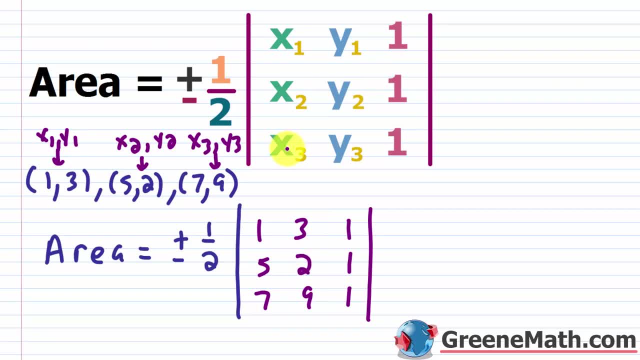 Plugging in for x sub 2, y sub 2.. That's how I got a 5 and a 2.. Plugging in for x sub 3, y sub 3.. That's how I got a 7 and a 9.. 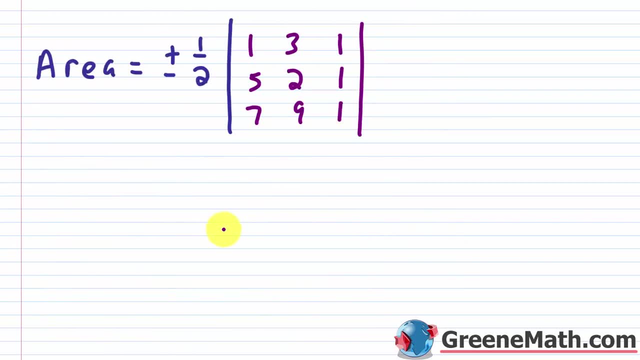 So let's copy this real quick. So how do I find the determinant quickly? Let's just copy this: 1, 3, 1.. 5, 2, 1, 7, 9, 1.. Again, the shortcut is to copy the first two columns. 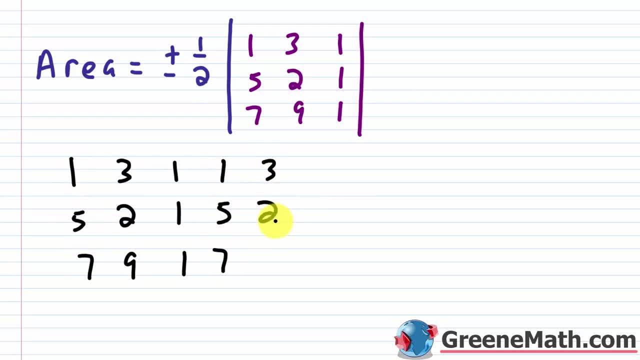 So you have 1,, 5,, 7,, 3,, 2,, 9.. And then you're going to start at this top left and multiply down this diagonal. 1 times 2 times 1 is 2.. And then, plus, you're going to multiply down this diagonal. 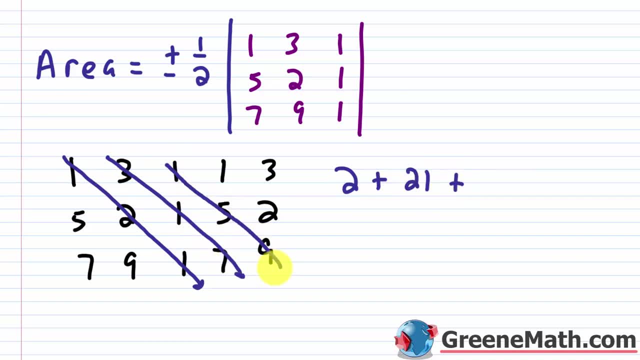 3 times 1 times 7 is 21.. And then, plus you're going to multiply down this diagonal, 1 times 5 is 5.. Times 9 is 45. If I sum that amount, 2 plus 21 is 23.. 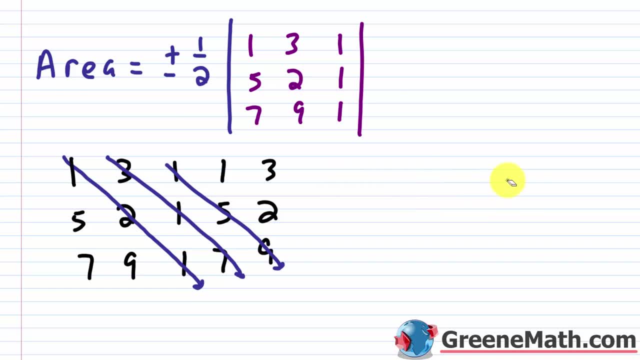 23. Plus 45 is 68. Okay, So the first part of this formula is 68. And then, for the second part, we're going to multiply up now. So, starting at the bottom left, I'm going to go up. 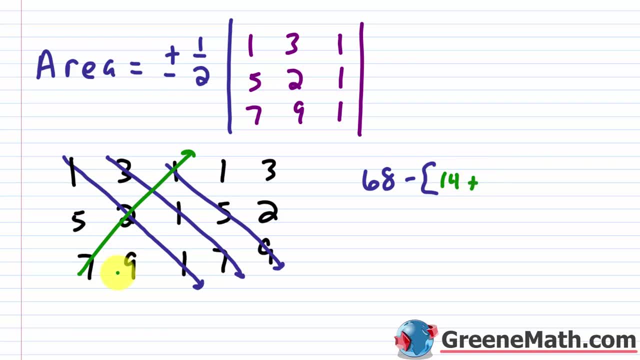 7 times 2 is 14.. Times 1 is still 14.. And then I'm going to multiply up 9 times 1 times 1 is 9.. Then, plus I'm going to multiply up 1 times 5 times 3 is 15.. 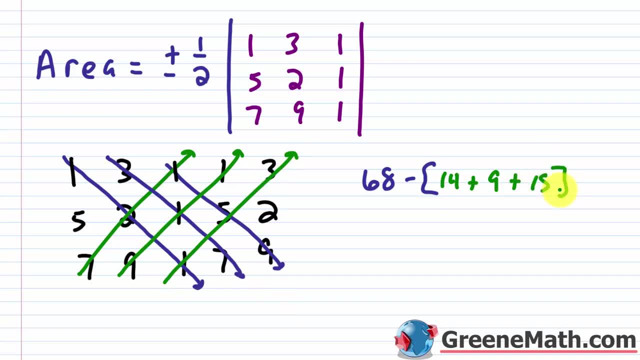 So 14 plus 9 is 23.. Plus 15 is 38. So you have 68 minus 38,, which is 4. 30. Okay, So the first part of this is that the determinant became 30. So the area- okay, the area is equal to in this case because we got a positive determinant. 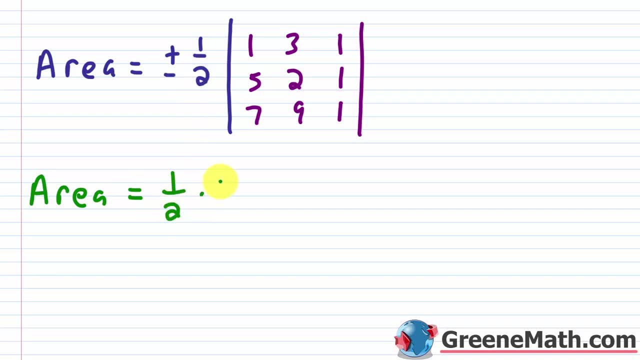 I'm just going to use the plus 1 half. So I'm just going to say 1 half times 30,, which is 15.. Now, when you work with triangles, remember your formula from basic geometry: 1 half times the base times the height. 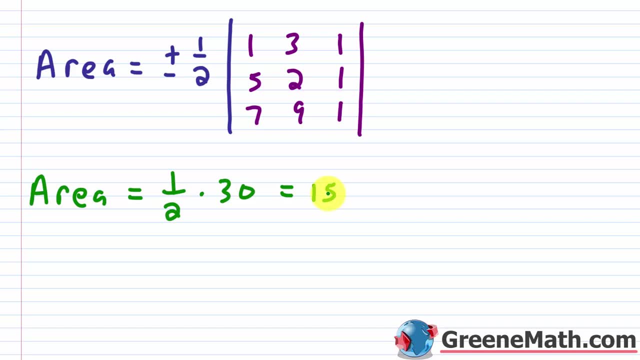 Remember, you have units involved with the base and the height, So you've got to think about the fact That's going to be square units. So if you were working with inches, it would be, you know, square inches or inches squared, or whatever that is. 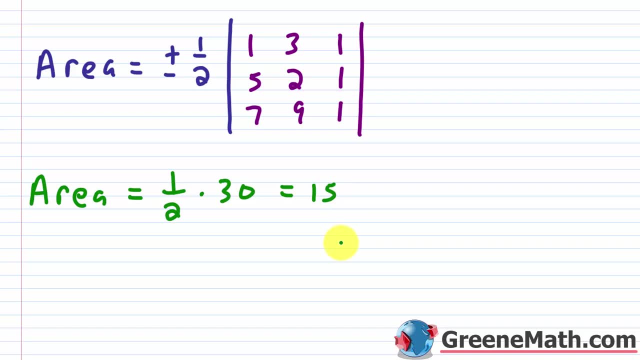 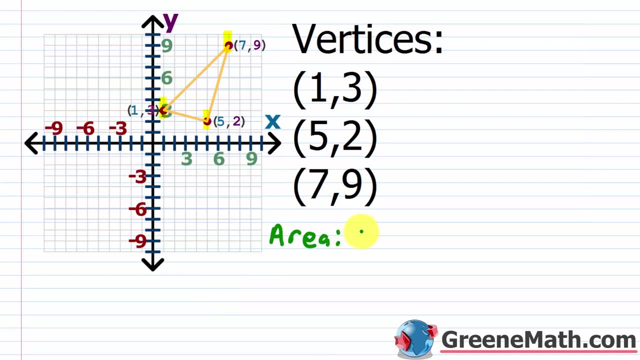 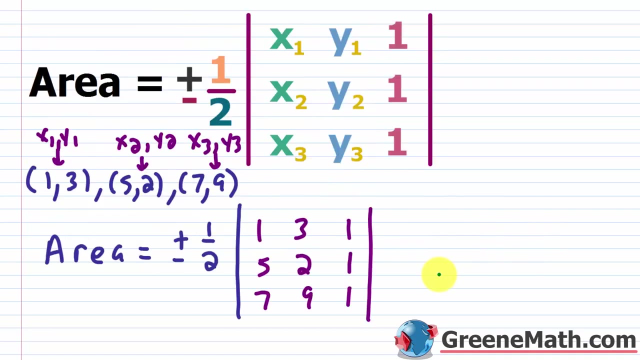 So you would really want to give a precise answer and say it's 15 square units. So I'll just say the area- And let me erase this- Is going to be 15 square. okay, square units. Now, really quickly, just to prove this to you, let's say I swap these two rows. 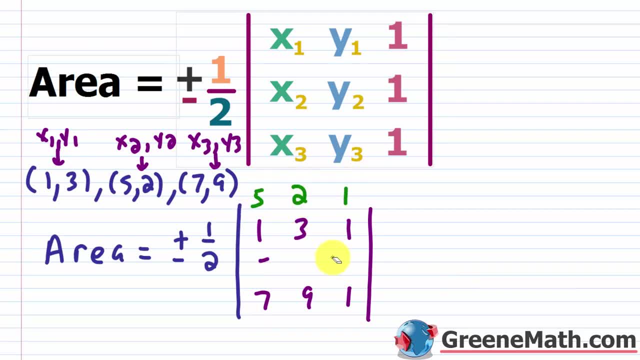 So let's say, I put 5,, 2, and 1 on the top. Erase that And I'll drag this up here. So really, this would correspond to what It would correspond to me choosing this point to be x sub 1, y sub 1, okay. 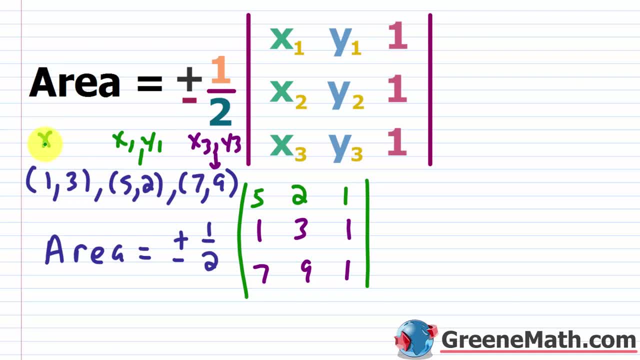 And this point to be x sub 2, y sub 2,. okay, And because I swapped two rows, the only effect this is going to have is it's going to change the sign of the determinant, right, So now the determinant is going to be negative 30.. 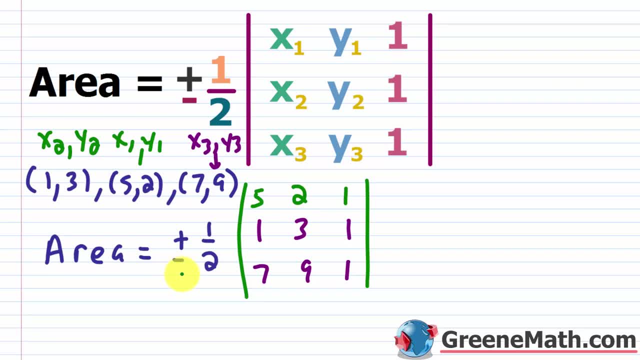 And so to get the area, I'm going to multiply by negative 1 half, And so I'm still going to, I'm going to get 15.. It's going to be 15 square units. But again, let me prove this to you real fast, because I know a lot of people say nope, you have to go in a certain order. 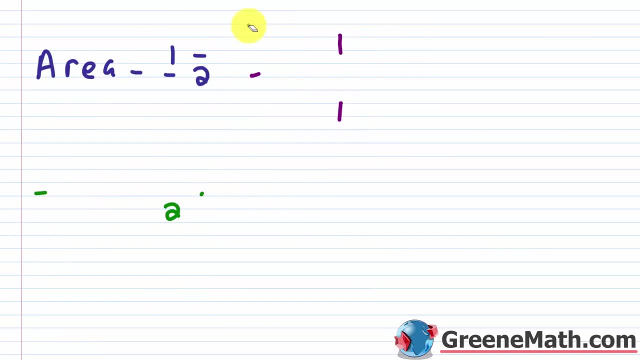 You do not, All right, So let me erase this And let me paste this in really quickly. So 5, 1, 7, 2, 3, 9, 1, 1, 1.. And again I'm copying the first two columns. 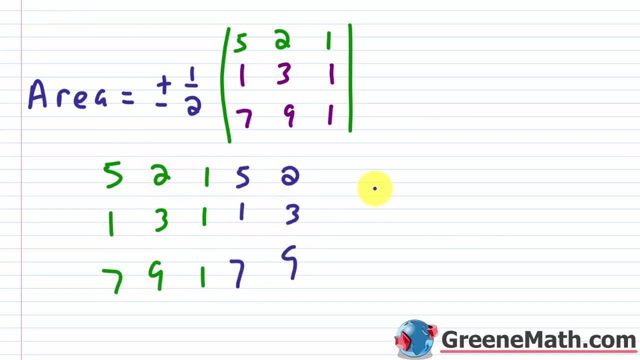 So 5, 1, 7, 2, 3, 9.. All right, So you already know the deal. We're going to start at the top left And we're going to multiply down 5 times. 3 times 1 is 15.. 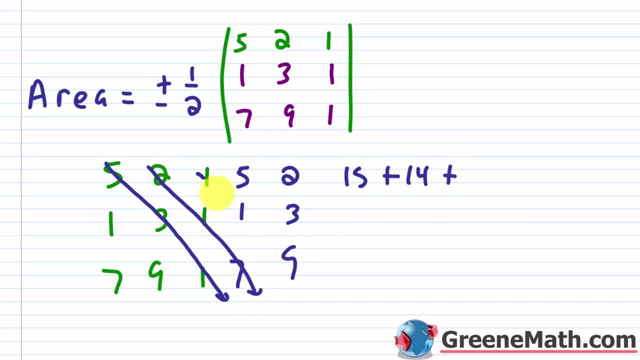 Then plus 2 times 1 times 7 is 14.. Then plus 1 times 1 times 9 is 9.. So you'll notice that this is 38. now, OK, And you're going to be subtracting away 68,, which is going to give you negative 30.. 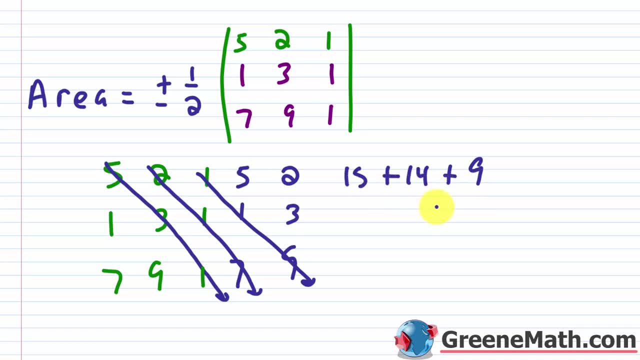 But let's go through it: 15 plus 14 is 29.. And then 29 plus 9 again is 38. OK, So this is 38. And then minus again. if we go up 7 times, 3 times 1 is 21.. 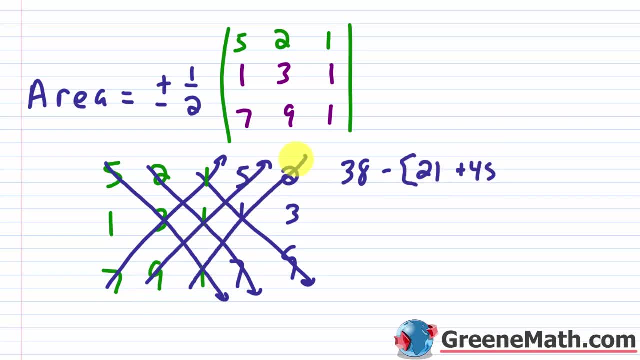 9 times 1 times 5 is 45.. OK, And 1 times 1 times 2 is going to be 2.. OK, 21 plus 45 is 66.. Plus 2 is 68.. Again, 38 minus 68 is negative 30.. 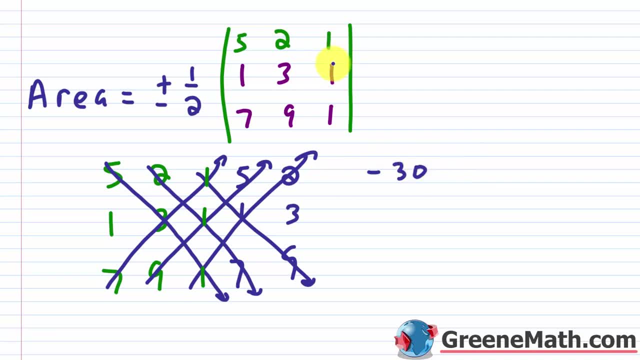 So again, I've just proved this to you, that swapping these two rows is basically like we've chosen different points, to be x sub 1, y sub 1, and x sub 2, y sub 2.. All I did was change the sign. 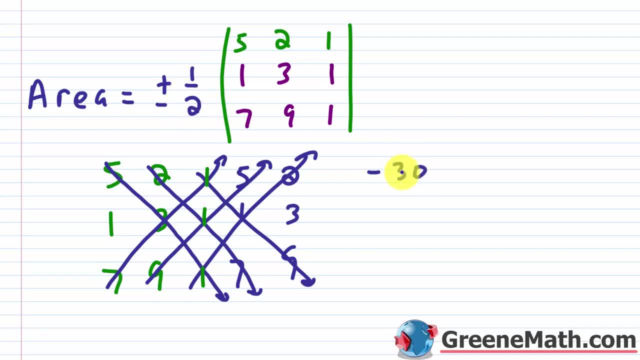 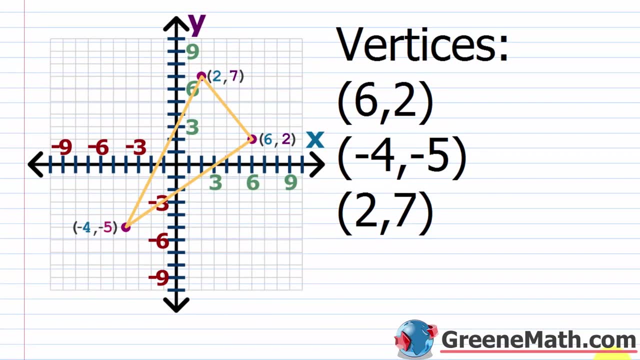 And I can now just multiply this by negative 1 half to get a positive 15.. And so, again, my answer for the area is 15 square units. OK, Let's just look at one more of these. It's a very, very easy concept. 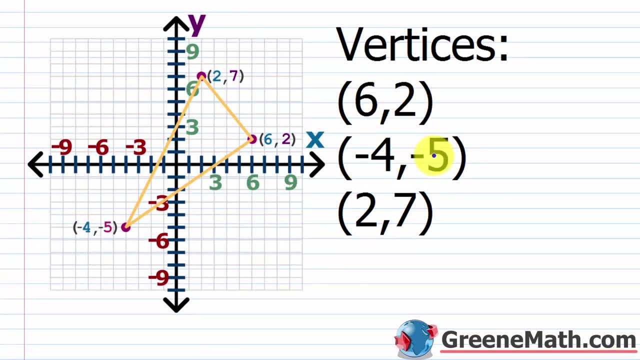 So the vertices we're given now is 6 comma 2, negative, 4 comma, negative 5, and 2 comma 7.. So here's your 6 comma 2.. Here's your 2 comma 7.. Here's your negative 4 comma, negative, 5.. 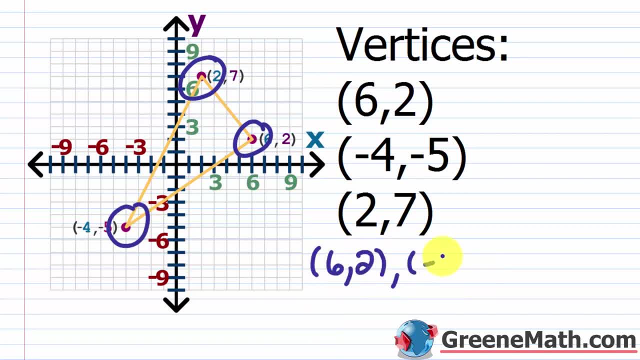 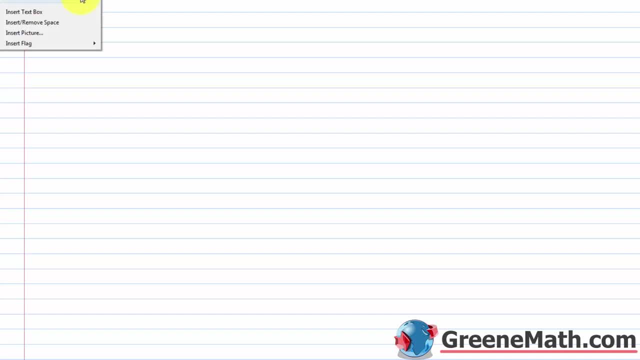 So let's copy those. You have 6 comma 2.. You have negative 4 comma, negative 5. And you have 2 comma 7.. OK, So let's copy this And let's just go to a fresh sheet. 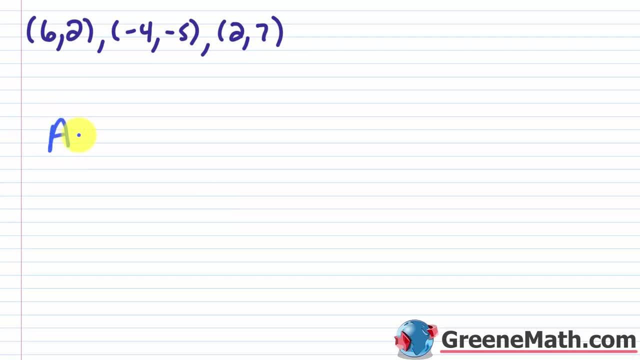 We should know the formula now. It's pretty easy. So the area is equal to 1 half And again, you've got that plus or minus out in front times, the determinant of let's go ahead and label this. So this I'm going to call x sub 1, y sub 1.. 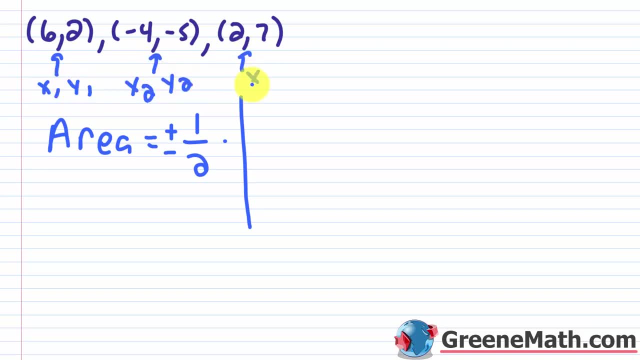 This I'm going to call x sub 2, y sub 2.. And this I'm going to call x sub 3, y sub 3.. So we know that the first row is coming from this right: The x sub 1, y sub 1.. 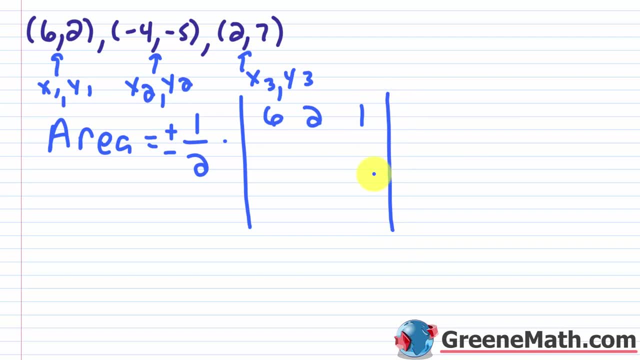 So 6 and then 2.. The last column, the third column, is always a 1.. So I can go ahead and just fill that in. Then this is x sub 2, y sub 2.. So negative 4 and then negative 5.. 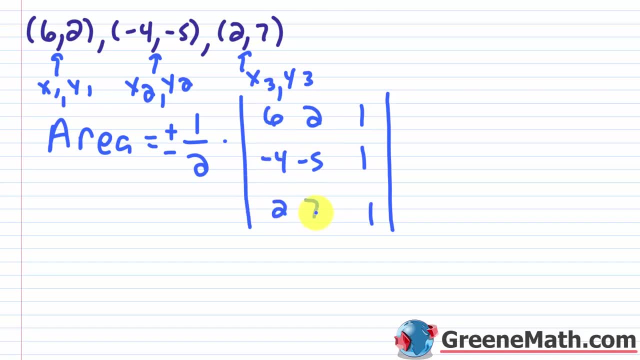 Then this is x sub 3, y sub 3.. So 2 and 7.. So very easy formula to remember. We don't need these points anymore. You just get rid of them. We're just going to take up space. 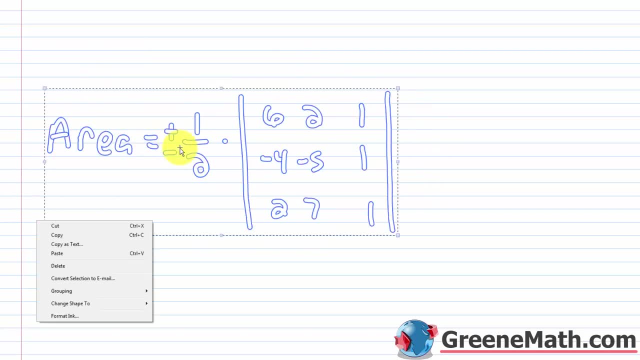 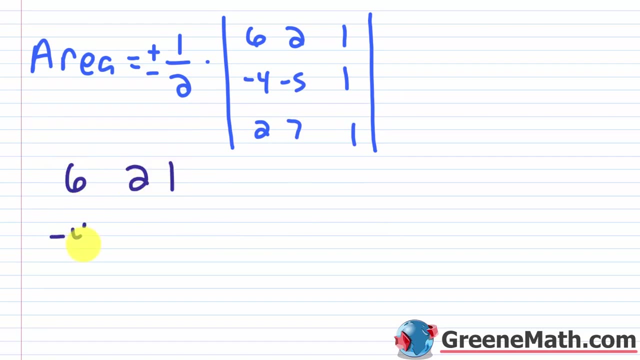 And let me get rid of that and slide this up out of our way And let me just copy our kind of matrix. So we have 6, 2 and 1, negative 4, negative 5 and 1, 2,, 7 and 1.. 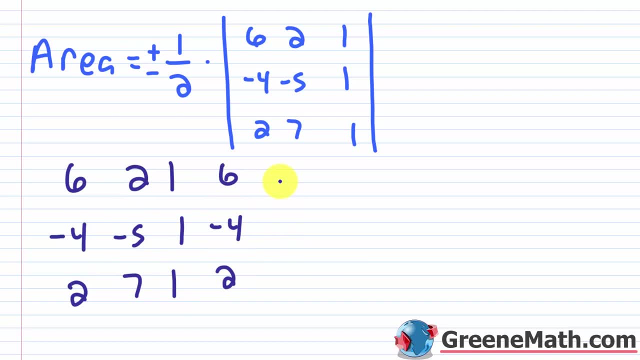 So copy the first two columns 6, negative 4 and 2.. And then 2, negative 5 and 1.. Negative 5 and 7.. So let's multiply again, starting from here and going down 6 times: negative 5 is negative 30. 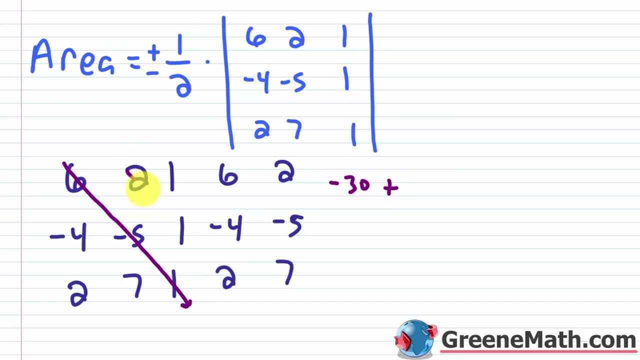 Times 1 is still negative 30. Then we're going to multiply down this way: 2 times 1 times 2 is 4.. Then this way: 1 times negative 4 times 7 is negative 28.. So we know that negative 30 plus negative 28 would be negative 58.. 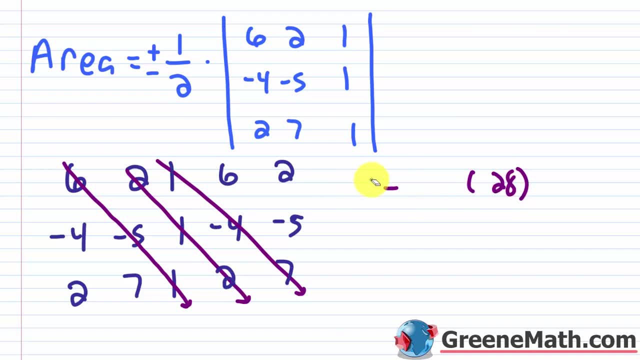 And negative 58 plus 4 would be negative 54. Okay, So the first part of this is negative 54. Then minus. Now we're going to go up, So we're going to start with negative 54.. We're going to start here. 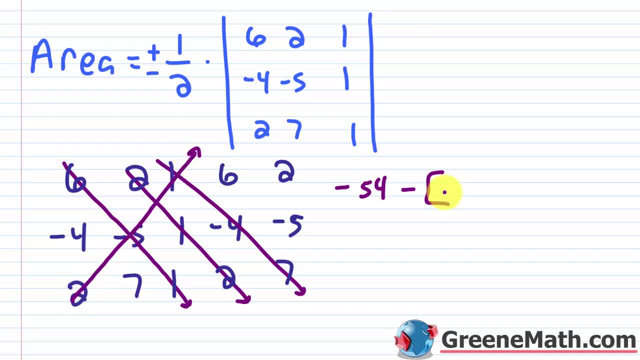 We're going to go 2 times negative, 5 times 1.. 2 times negative, 5 is negative 10.. And then times 1 is obviously still negative 10.. 7 times 1 times 6 is going to be 42.. 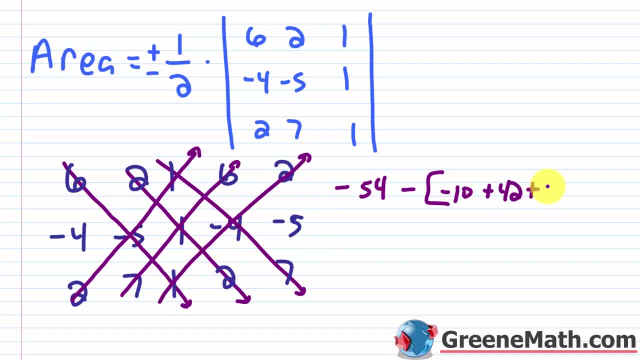 And then we have 1 times negative, 4 times 2, which would be negative 8.. Okay, So negative 10 plus negative 8 is negative 18.. So what is negative? 18 plus 42?? That's going to give me positive 24.. 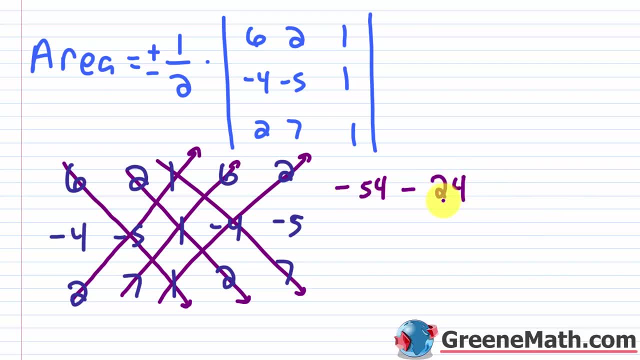 Okay, So what you have here is negative 54 minus 24.. Which is negative 78. Okay, So, negative 78. So let me erase this. The value of the determinant of this guy is negative 78. So our area will be equal to: because it's negative, you're going to use the negative 1 half. 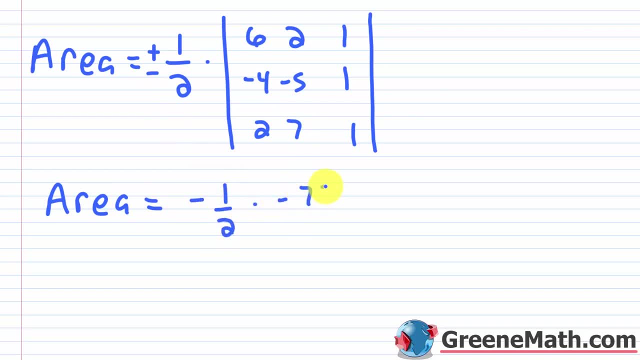 So negative 1 half times your negative 78.. Okay, So what is that going to give us? Well, forget about the sign, because we know it's going to be positive. 78 divided by 2 is 39. So this equals 39.. 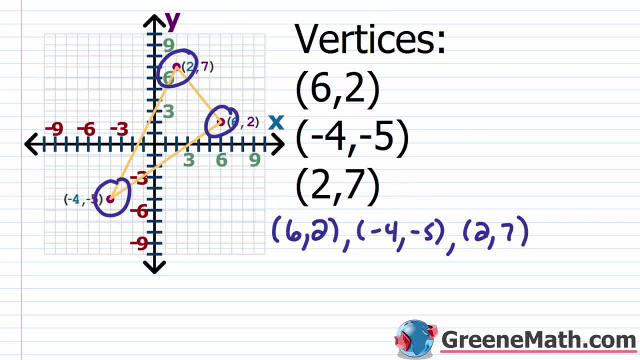 And again, when you write your answer, you want to put square units. So let's just erase this And we'll say that the area is 39 square units.